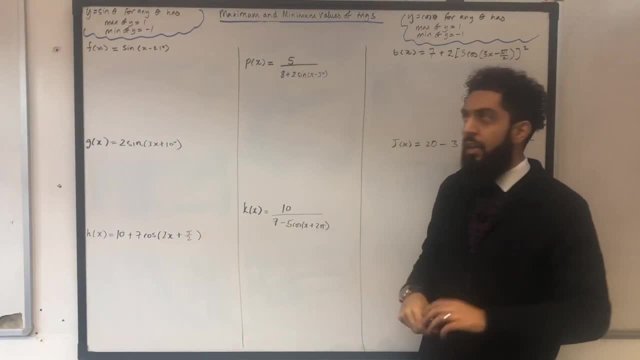 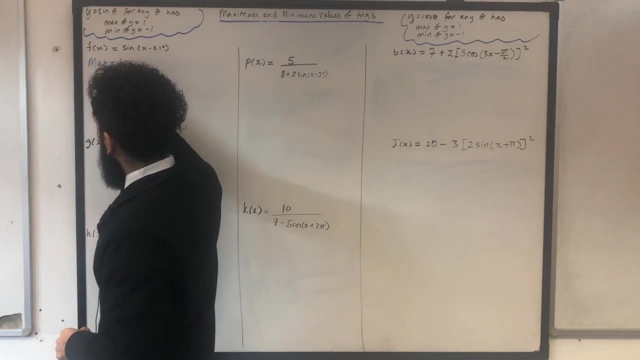 The angle can change, but the maximum and minimum will remain the same. So the maximum of this particular function is 1, and the minimum of this particular function is minus 1.. In the exam you could be asked to work out the smallest positive value of x for which the function 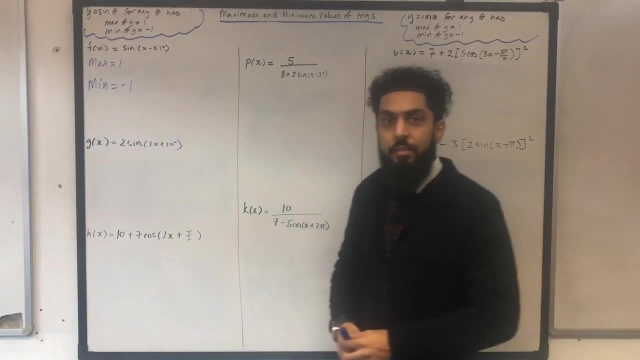 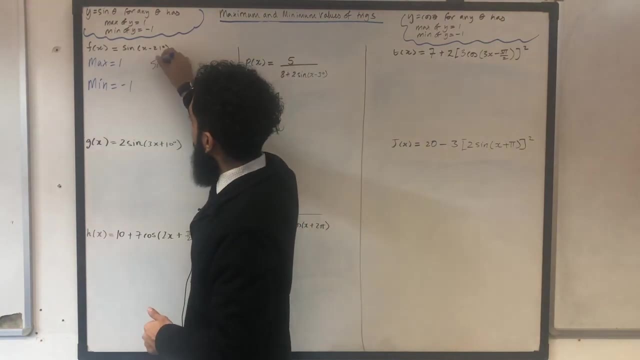 f of x has a maximum- in this case 1, and a minimum, in this case, minus 1.. You have to solve the following equations: For the maximum, you have to solve: sine in bracket x minus 21 degrees. Now the function f of x, which is equal to 2, sine in bracket 3x plus 10 degrees. For the: 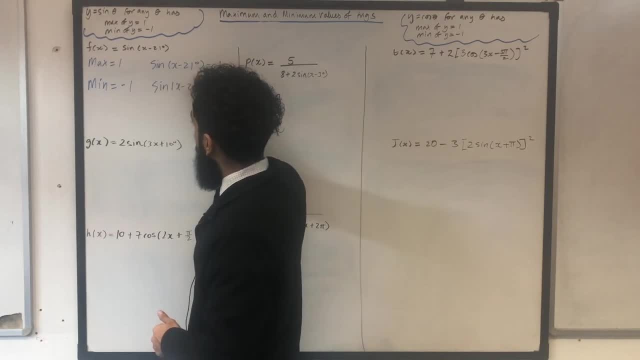 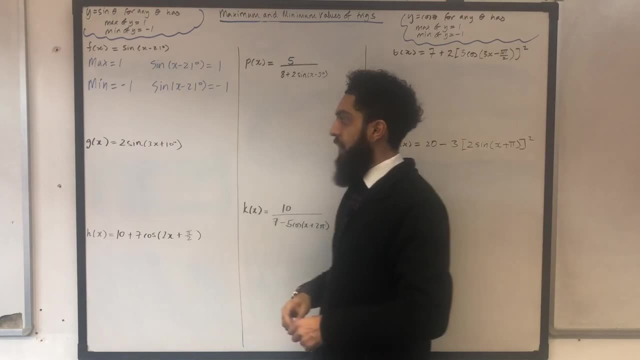 minimum you have to solve: sine in bracket x minus 21 degrees equals minus 1.. Now next function g of x, which is equal to 2 sine in bracket 3x plus 10 degrees. Okay, I could be asked to work out. 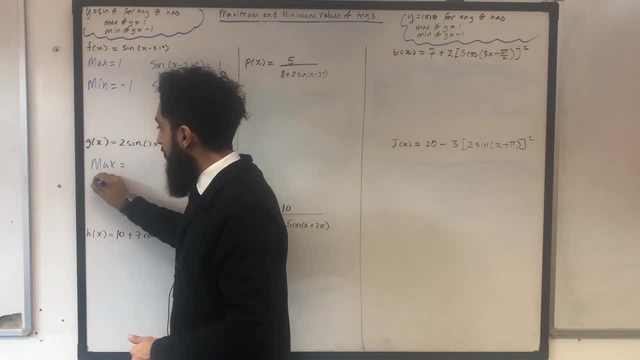 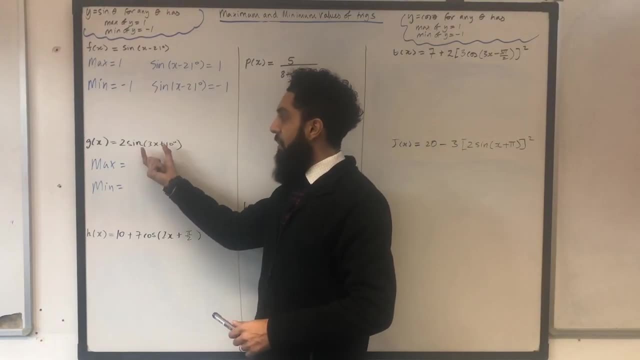 the maximum value of this particular function and the minimum value of this particular function. Well, to maximize g of x, I need to maximize my sine, and the maximum value of sine will just be 1, so the maximum value of g of x squared is equal to 2.. So the maximum value of sine will just be 1,. 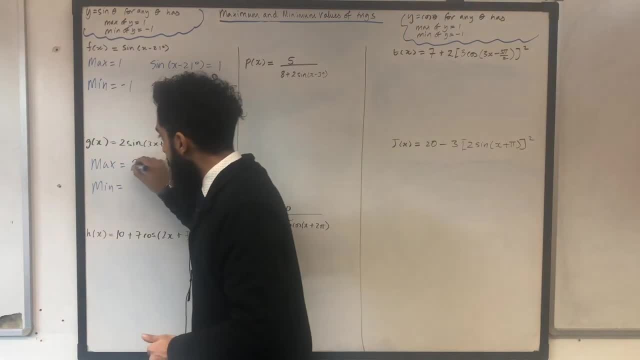 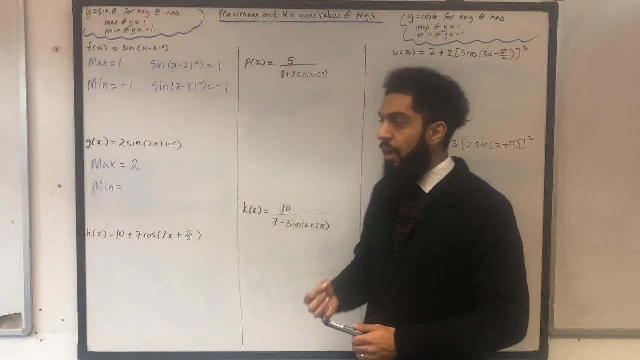 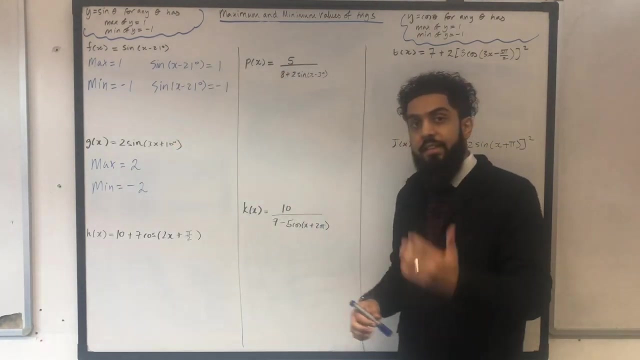 of g of x is 2 times 1, which is just 2.. To minimize the function g of x I need to minimize my sine, and the minimum of sine is minus 1. hence the minimum of g of x is 2 times minus 1 minus 2.. In the exam I could be asked to work out the smallest. 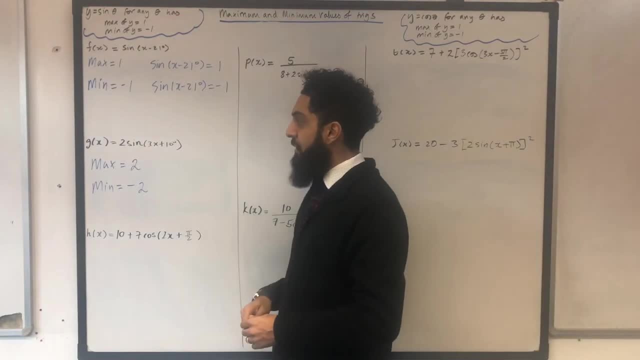 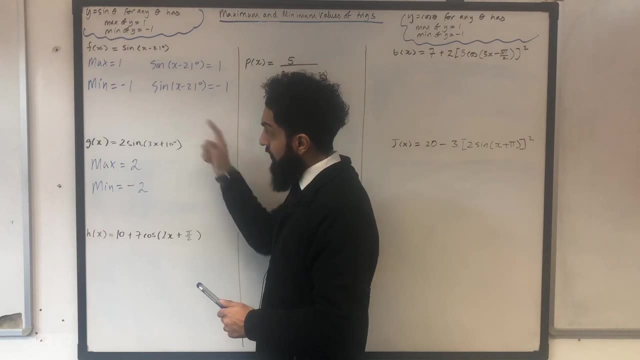 positive value of x for which the function g of x has a maximum- in this case 2- and a minimum, in this case, minus 2.. So to find the smallest positive value of x for which the function g of x has a maximum of 2, I need to solve the. 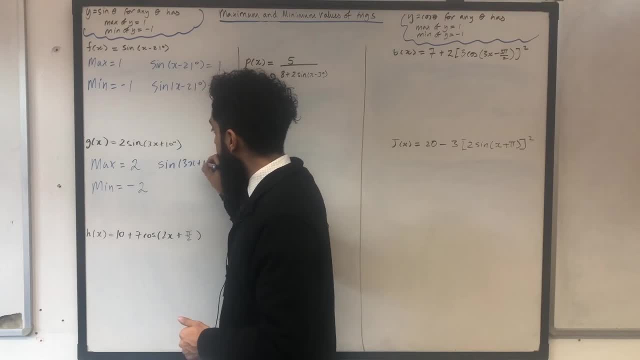 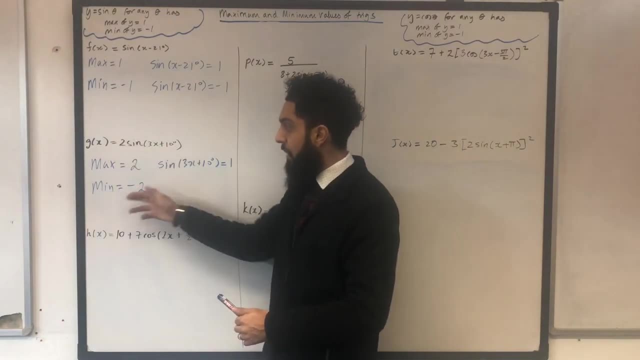 equation sine in bracket 3x plus 10 degrees equal to 1.. To work out the smallest positive value of x, for which the function g of x has a minimum of minus 2, I need to solve the equation sine in bracket 3x plus 10 degrees equal. 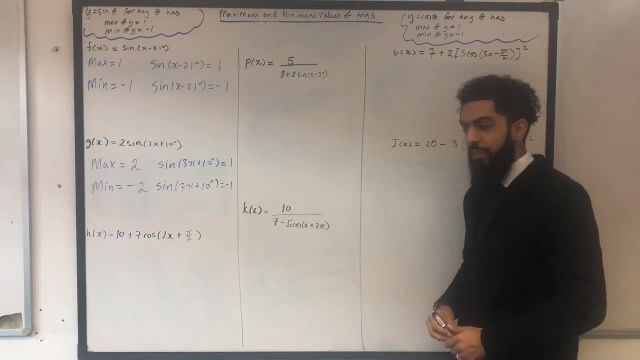 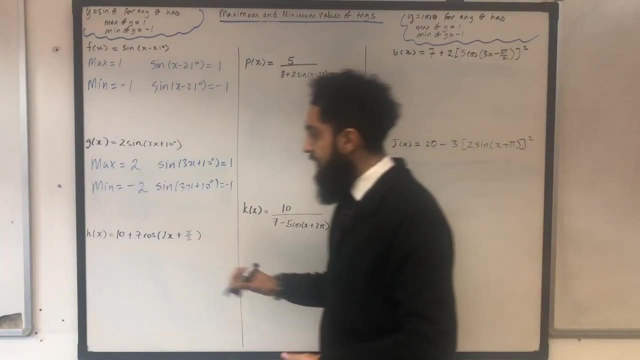 to minus 1.. Right, the next function: h of x equal 10 plus 7, cos in bracket 2x plus pi over 2.. What I want to do is to solve the equation: sine in bracket 3x plus 10 degrees equal to 1.. So what I want to do is work out the maximum value of this function and 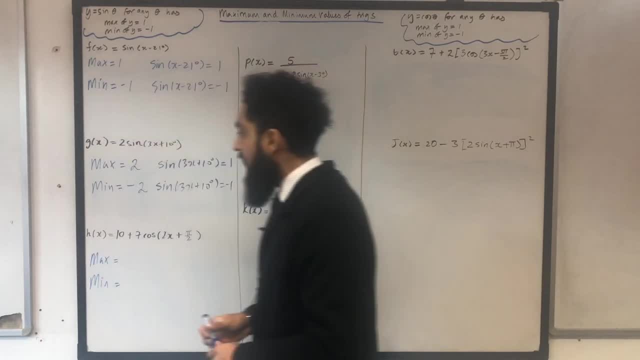 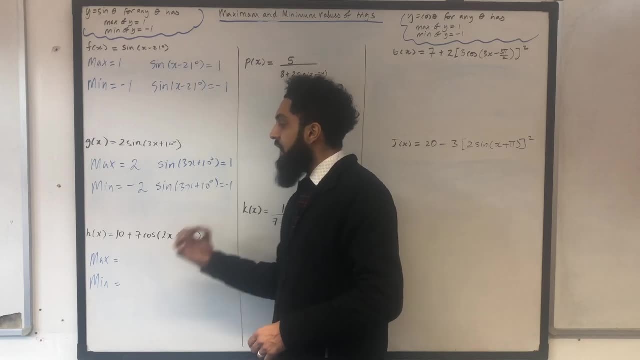 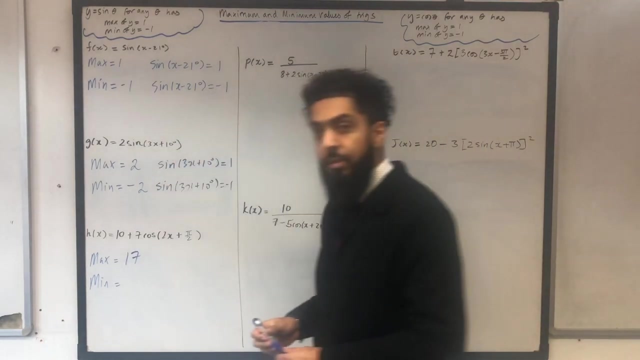 the minimum value, Okay. so if I want to maximize the function h of x, I need to maximize my cos. okay, and the maximum of cos is just 1. so I have 10 plus 7 times 1, which is 10 plus 7, which is 7t. To minimize the function h of x, I need to. 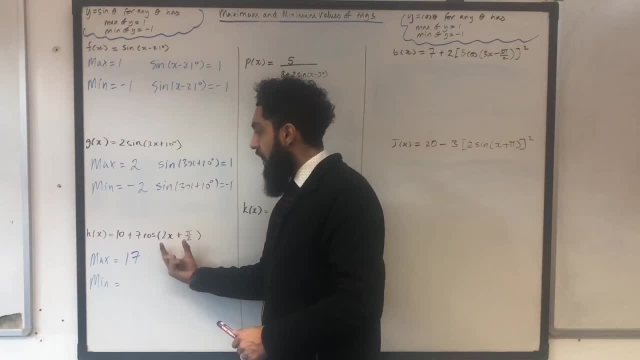 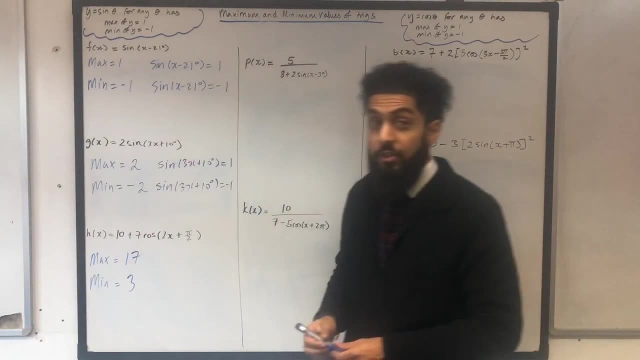 minimize my cos and the minimum of cos is minus 1. so 10 plus 7 times minus 1 is minus. 1, is 10 minus 7, which is 3.. In the exam I could be asked to work out the smallest positive value of x for which the function h of x has a maximum in. 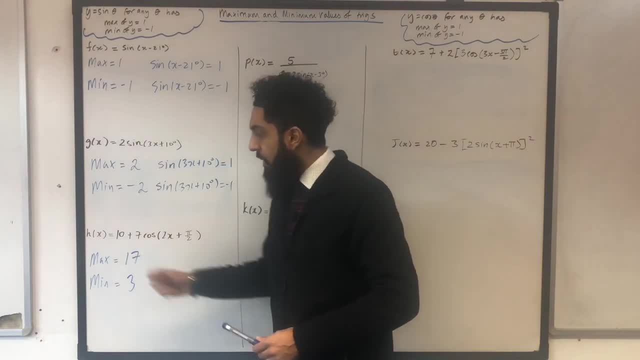 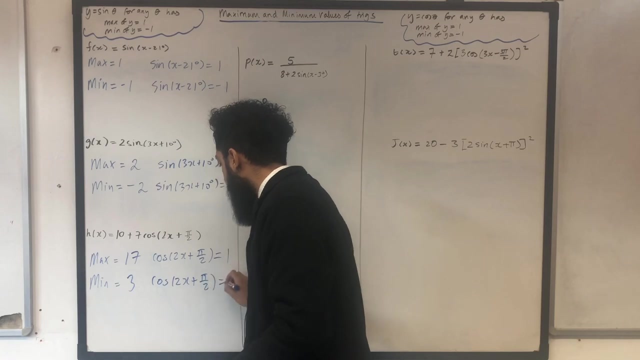 this case, 17, and minimum in this case 3.. For the maximum, I need to solve the equation cos in bracket 2x plus pi over 2, equal to 1.. For the minimum, I need to solve the equation cos in bracket: 2x plus pi over 2, equal to minus 1.. 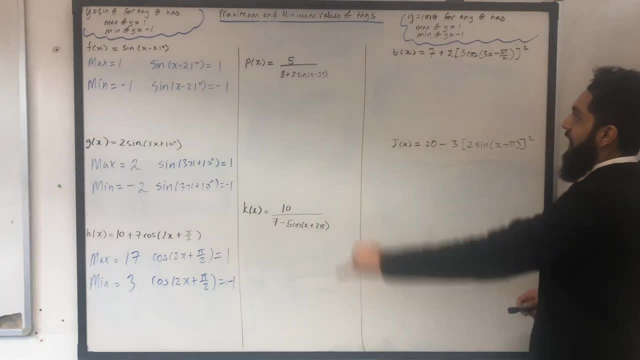 Let's move on to the next crispy function. Now I've got function t of x, which is equal to 7, plus 2 square brackets, 3 cos in bracket 3x minus 3 pi over 2 square bracket squared. Now the power 2 makes things extremely. 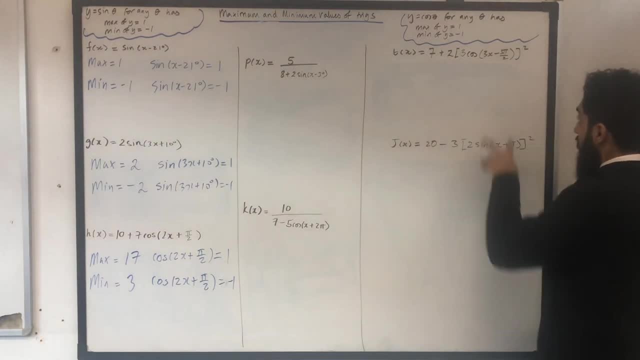 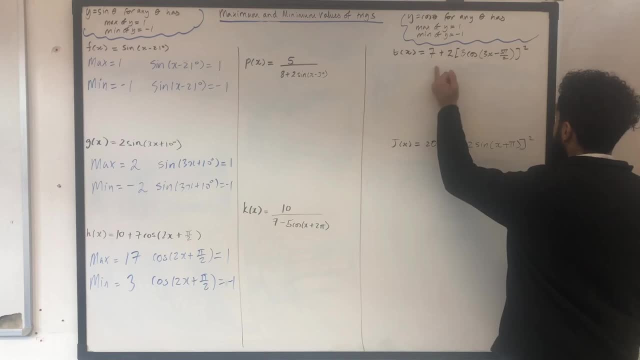 3 is 18.. 18 plus 7 is 25.. In the same way, if I replace the cos with minus 1,, 3 times minus 1 is minus 3.. Minus 3 squared is 9.. 9 times 2 is 18.. 18 plus 7 is 25.. 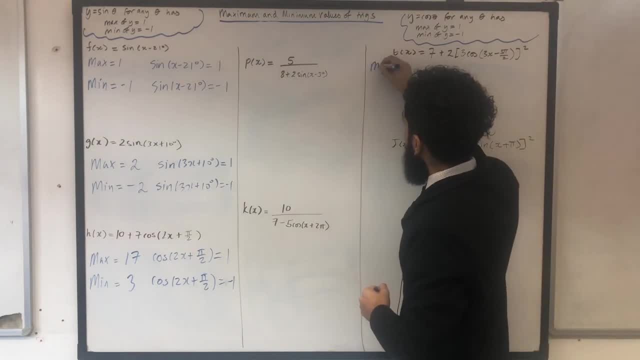 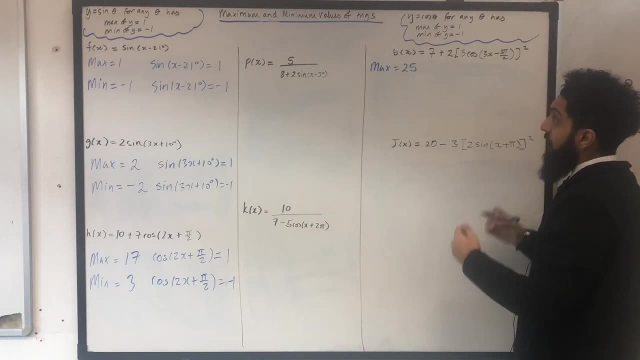 The maximum value of t of x will be 25.. In the exam, I could be asked to work out the smallest positive value of x for which the function t of x has a maximum, in this case 25.. This time I'm going to be solving. 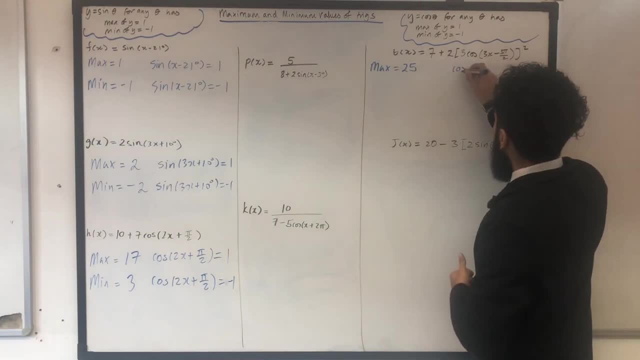 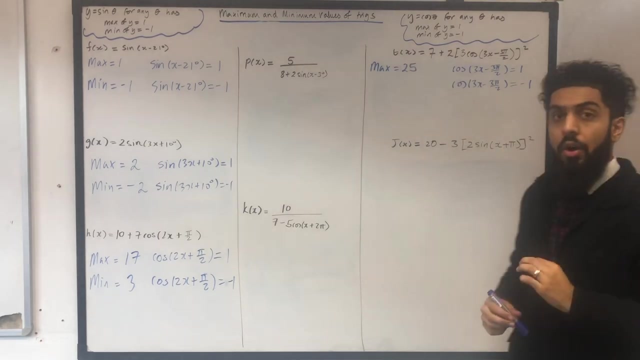 two equations, and the two equations that I solve are: cos in bracket 3x minus 3 pi over 2, equal to 1, and cos in bracket 3x minus 3 pi over 2, equal to minus 1.. Once I solve these two equations, I take the smallest positive value of x. Ok, right now I 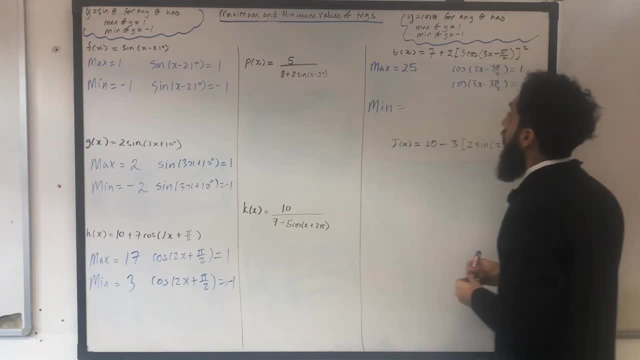 want to work out the minimum value of the function t of x. Well, to minimise the function t of x, I need to set the cos equal to 0.. So 3 times 0 is 0, zero squared is 0. times 2 is 0 plus 7 is 7. so the minimum value of the 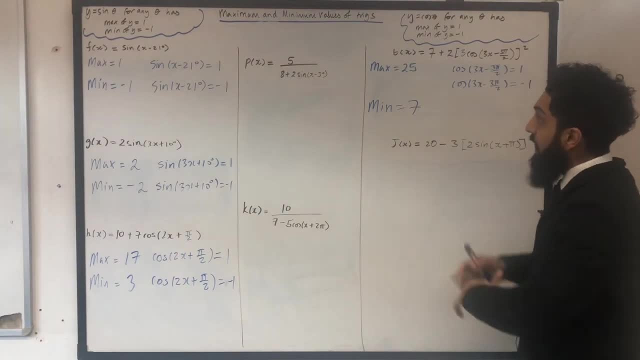 function t of x is 7.. Ok, in the exam I could be asked to work out the smallest positive value of x for which the function t of x has a minimum, in this case 7.. So I need to solve the equation: cos in bracket 3, x minus 3 pi over 2 equal to 0. Okay, nice. 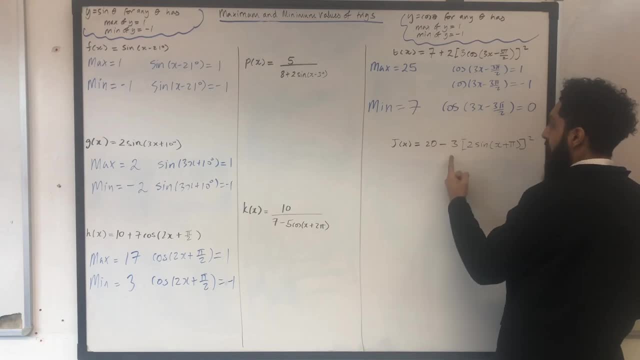 Now I've got the function g of x equal 20 minus square bracket 2. sine in bracket x plus pi, square bracket squared. Again I've got a power 2. I need to be careful. My first observation is: if I replace the sine with 1 or minus 1, I will end up with 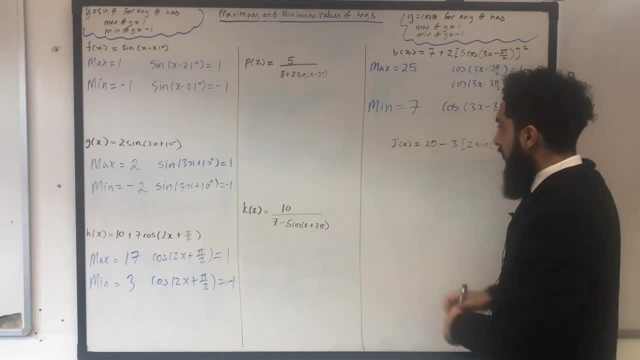 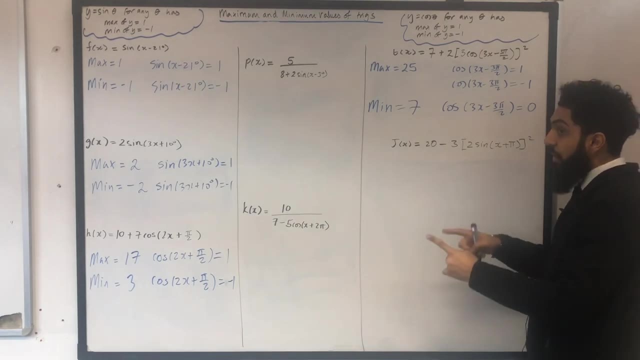 an output of 8.. Okay now, if I replace the sine with 0, I will end up with an output of 20.. Now, 20 is more than 8, so the maximum value of g of x is equal to 20.. In the exam I could be: 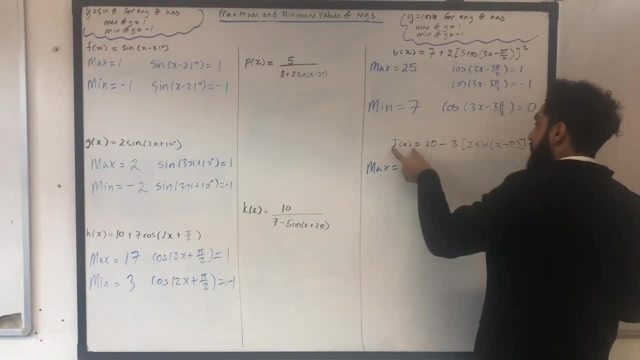 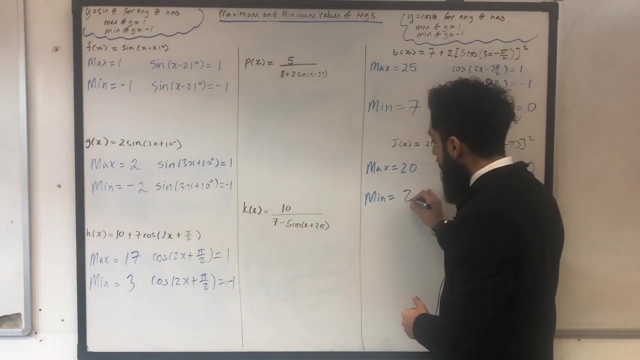 asked to work out the smallest positive value of x, for which the function g of x has a maximum value of 20.. I need to solve the equation sine in bracket: x plus pi equal to 0.. Right, the minimum value of the function g of x is equal to 8.. I could be asked in the exam to work out the smallest. 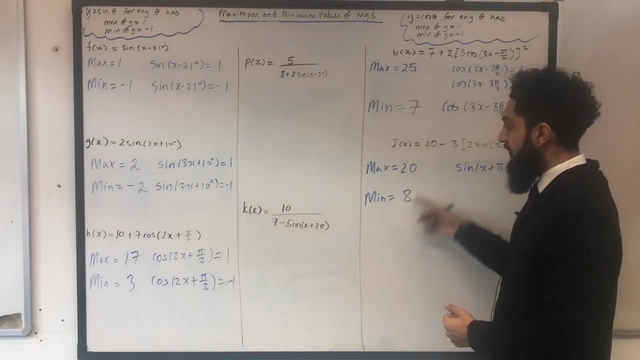 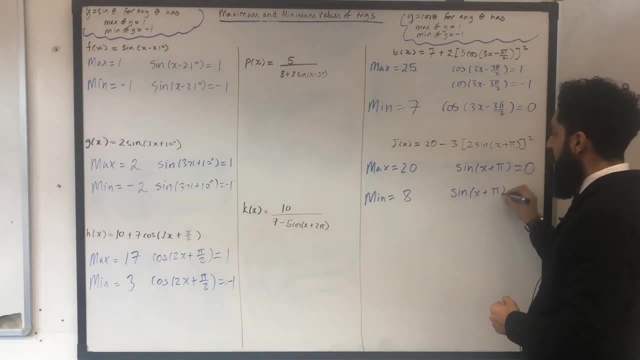 positive value of x, for which the function g of x has a minimum, in this case 8,. I need to solve two equations, And those two equations are: sine in bracket x plus pi, equal to 1,. sine in bracket x plus pi. 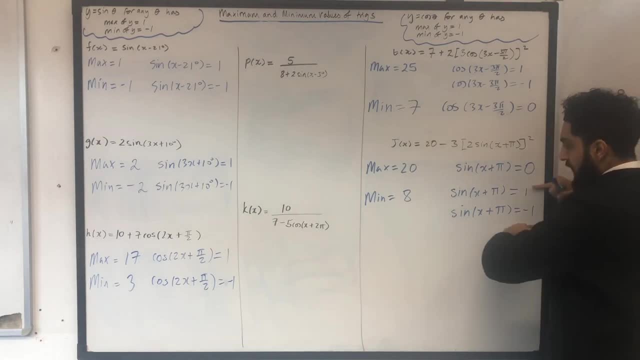 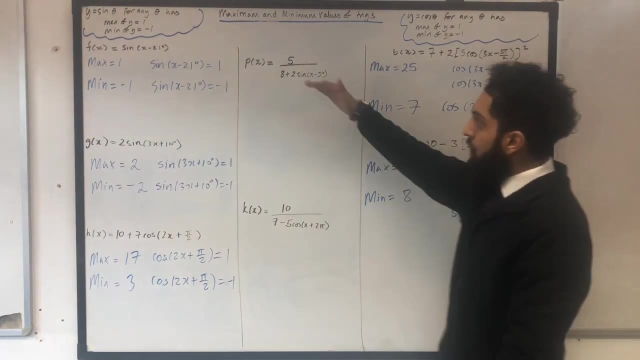 equal to minus 1.. So I solve these two equations and then take the smallest positive value of x. Okay, right, moving on to the last two functions: p of x and k of x are both in fraction form. something very juicy happens when you have a function in fraction form. I'm going to start. 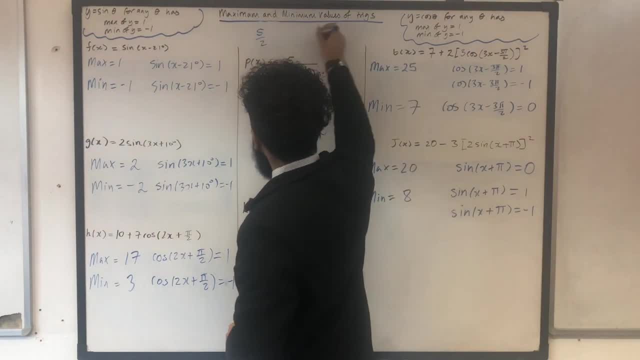 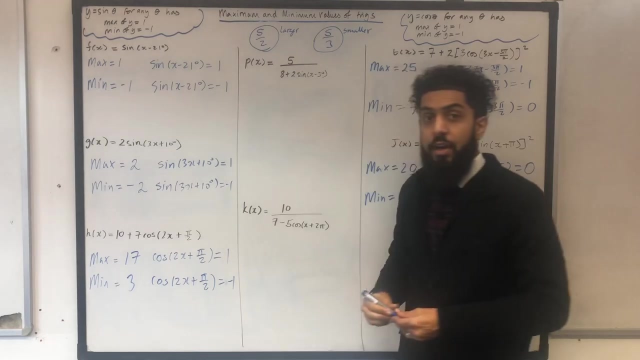 off with two fractions: 5 over 2 and 5 over 3.. I want to compare these fractions. Well, first of all, I can see that 5 over 2 is larger and 5 over 3 is smaller. The reason why 5 over 2 is larger: 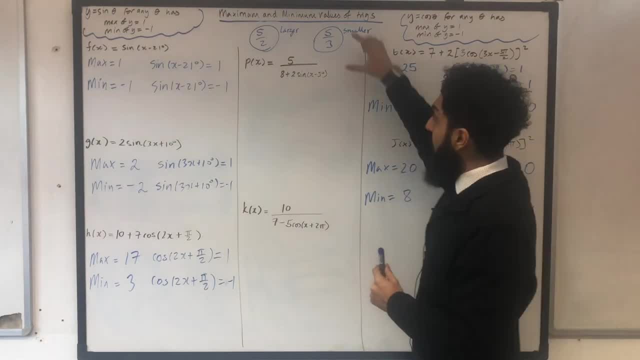 is because the denominator is smaller. The reason why 5 over 3 is smaller? because the denominator is smaller. The reason why 5 over 3 is smaller is because the denominator is smaller. The reason why 5 over 3 is larger is because the denominator is larger. So, in general, if you have a 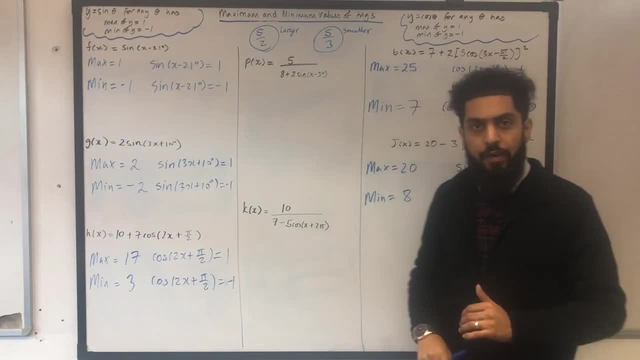 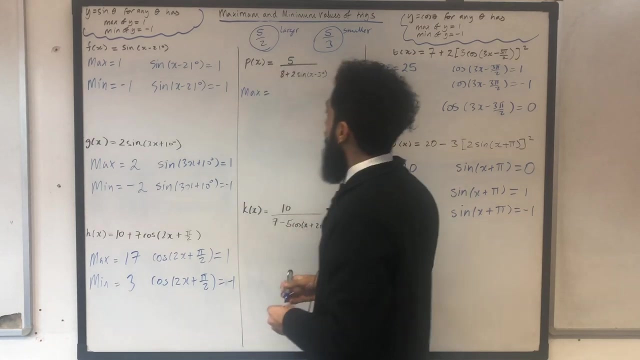 function in fraction form. to maximise the function, what you have to do is minimise the denominator. Okay, to minimise the function, you have to maximise the denominator. So let's first of all work out the maximum of p of x Right to find the maximum of p of x, which is this fraction. 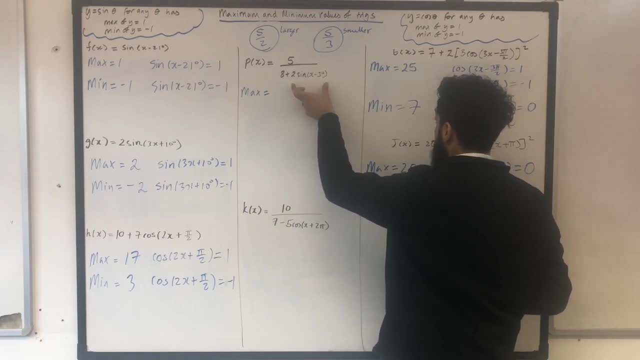 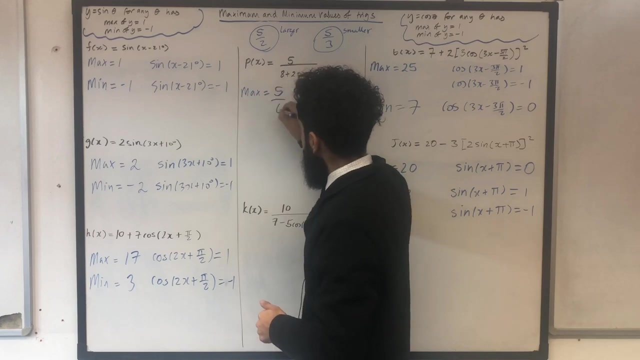 I need to minimise the denominator. To minimise the denominator, I need to minimise the sign. Okay, so the sign will be minus 1.. I will get 5 over 8 plus 2 times minus 1, which is 5 over 6.. Now I want to work out the minimum of this function. Well, to minimise p of x. 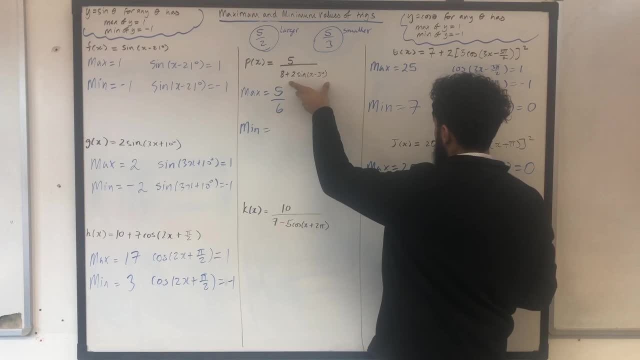 which is this fraction, I need to maximise the denominator. To maximise the denominator, I need to maximise the sign. So I replace the sign with 1.. I get 5 over 8 plus 2 times 1, which is minus 1.. 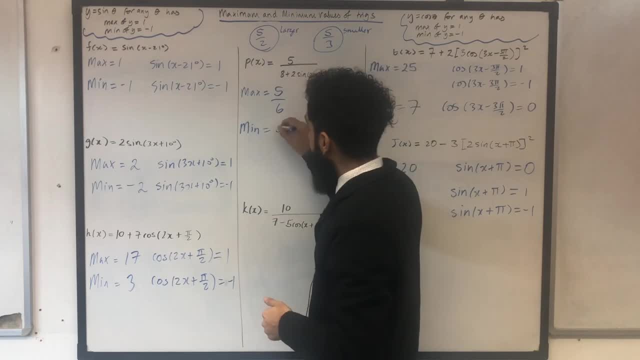 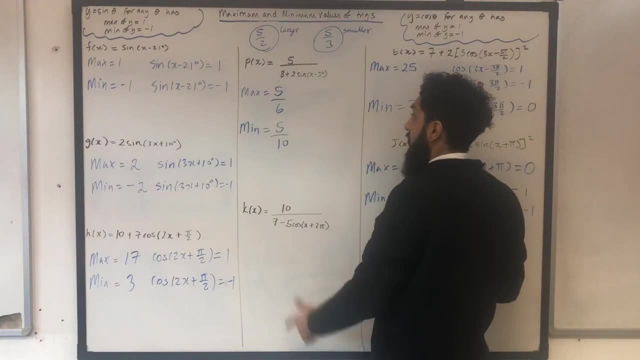 Now I can just write 5 over 10.. Now in the exam I could be asked to work out the smallest positive value of x for which the function p of x has a maximum, in this case 5 over 6.. All I need to do 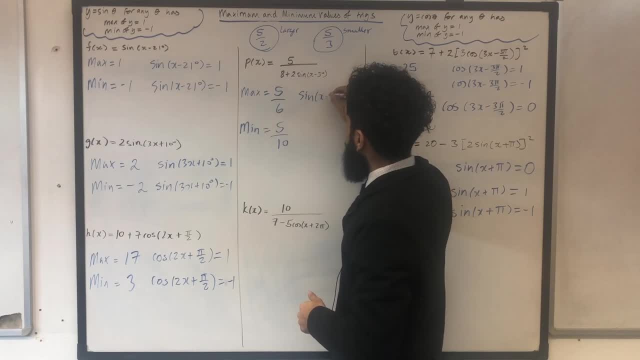 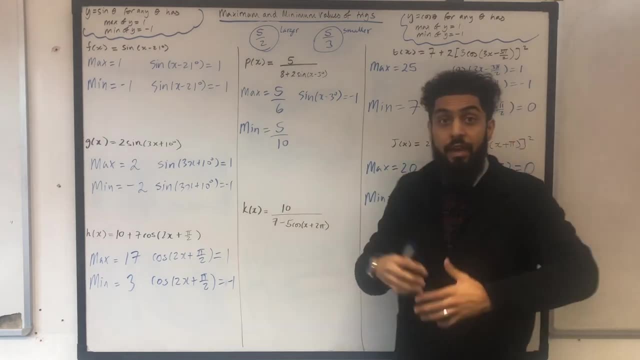 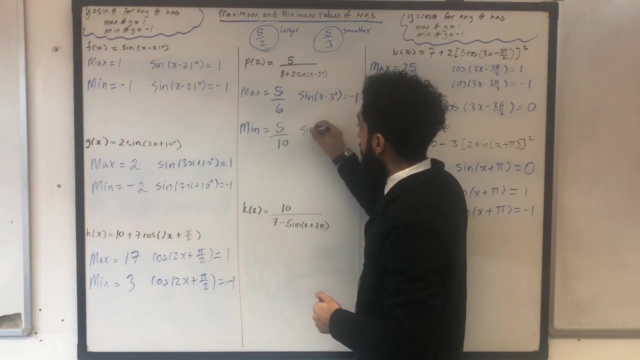 is solve the equation sign in bracket x minus 3 degrees is equal to minus 1.. In the exam I could be asked to work out the smallest positive value of x for which the function p of x has a minimum, in this case 5 over 10.. I need to solve the equation. sign in bracket x minus 3 degrees is.